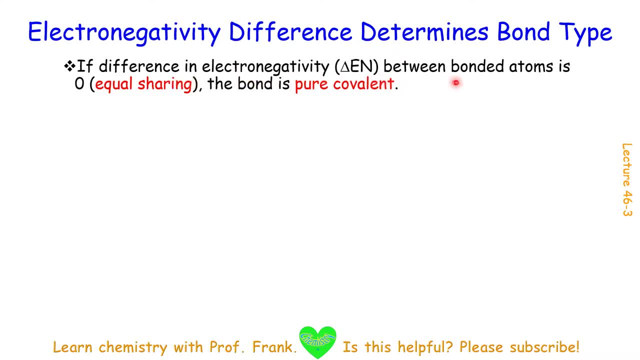 If the difference in electronegativity between bonded atoms is zero, equally shared, then the bond is pure covalent. If the data En is 0.1 to 0.4, the bond is non-polar covalent. 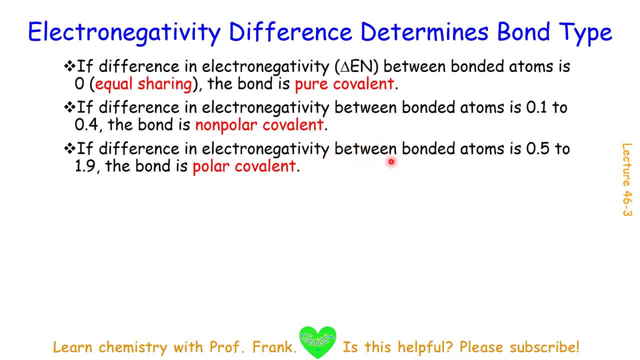 However, if the data Hen between bonded atoms is 0.5 to 1.9, the bond is non-polar covalent. It is classified as a polar covalent bond. If the difference in electronegativity is larger than or equal to two, the bond is ionic. 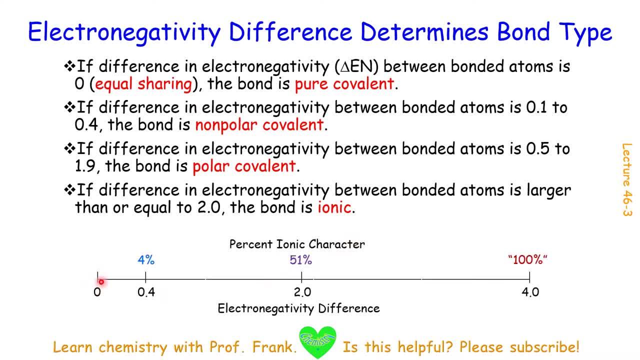 Right here there is a pure covalent bond Between data En of 0.1 to 0.4,. the bond is non-polar covalent between data En of zero to 0.5 is non-polar covalent. 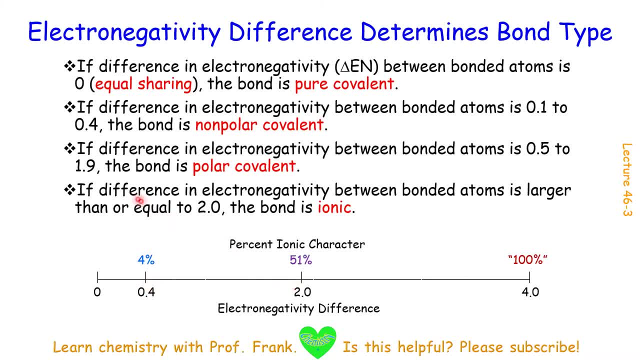 n of 0.4 to 1.9, we call that bond polar covalent. If the electron activity difference is 2 or higher, then the bond is ionic bond And here shows the percent ionic character: Non-polar. 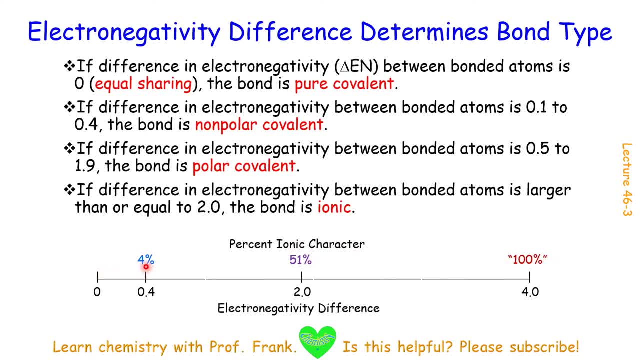 covalent bond have 4% or less of ionic character. Polar covalent bond have somewhere between 0.4 to close to 50% of ionic character, And if that HEN is 2.0, then the percent of ionic. 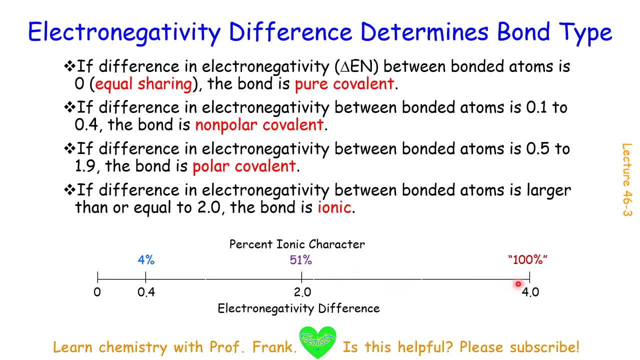 character is 51.. If the difference is 4.0, then that bond has 4.0.. So if the difference is 4.0, then that bond has 4.0.. So if the difference is 4.0, then that bond has 4.0.. 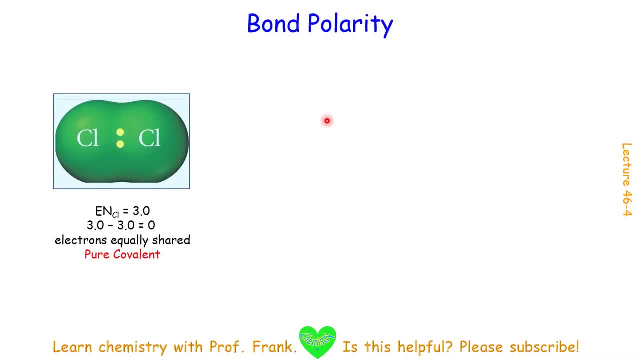 So if the difference is 4.0, then that bond has 100% ionic character. Now let's take a look at bond polarity, Chlorine molecule. even though the electron activity value for chlorine is pretty high- 3.0,- but the difference in electron activity is 0.. Therefore, electrons 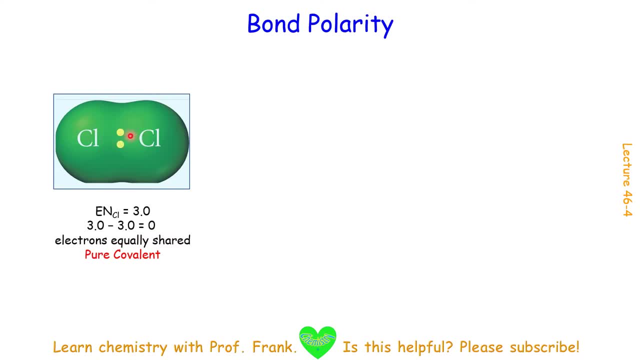 those two electrons are equally shared by the two chlorine atoms. We call this bond. we call this Cl- Cl bond, pure covalent. The shared electrons in hydrogen chloride molecule is, however, not equally shared. Those shared electrons, they are pulled. 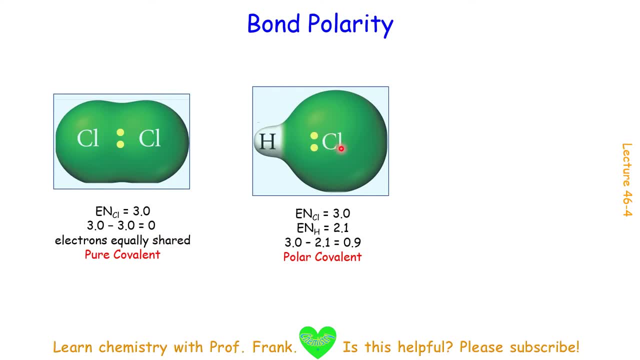 much closer to the chlorine atom. The electron activity difference is 0.. So the difference is 0.9. That's within 0.5 to 1.9.. That's why this HCl bond is polar covalent. 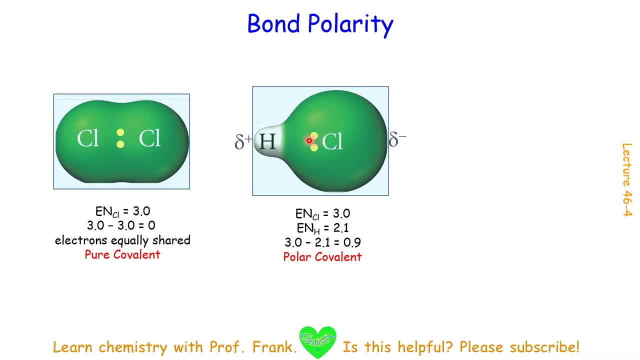 If it's polar covalent, the molecule should have two different ends. One side is negative, partially negatively charged, and the other side is partially positively charged. So we can also use this notation to show the partially positive end and the partially negative. 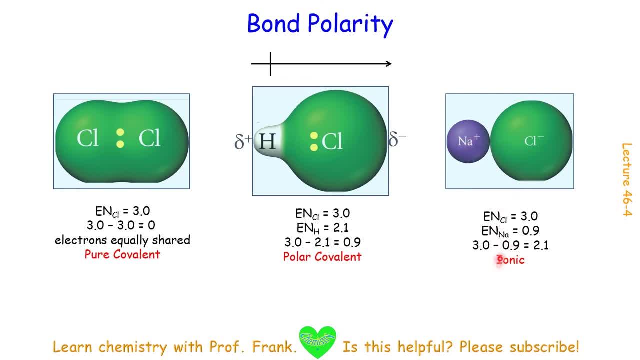 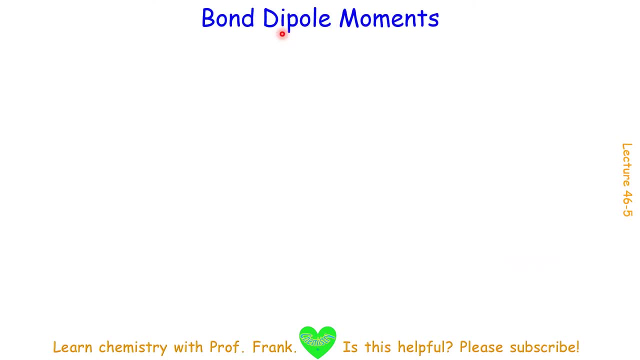 end, And here that's an ionic compound. The difference in electron activity is 2.1.. Now we are going to take a look at dipole moments. Dipole moment is a quantitative way of describing the polarity of electrons. We know that dipole moments are the polarity. 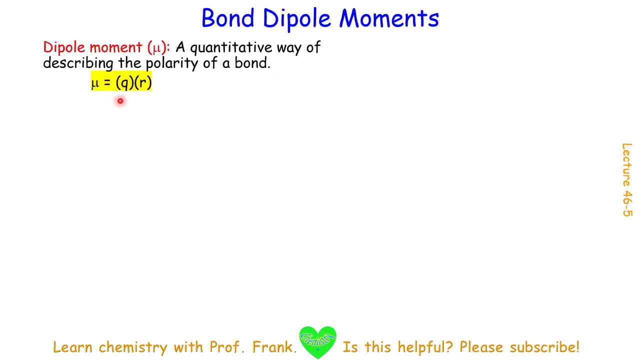 of electrons And dipole moments are the polarity of electrons, So we can use this of a bond. it can be calculated by the product of charge on the distance between two bonded atoms. The r is literally the bond length. The unit for dipole moment is divided. Therefore, 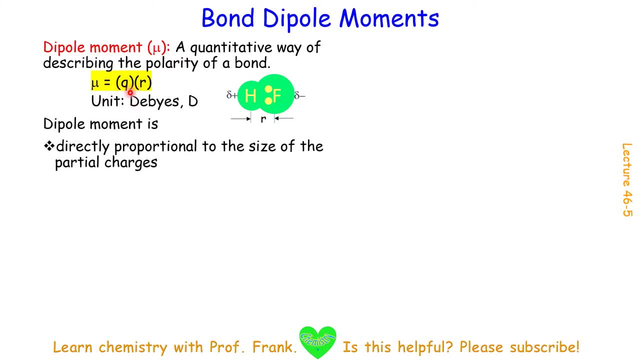 the dipole moment is directly proportional to the size of the partial charges, Q, also directly proportional to the distance between the two atoms or the bond length. And the dipole moment is also directly related to data n here Here I show us a few examples. 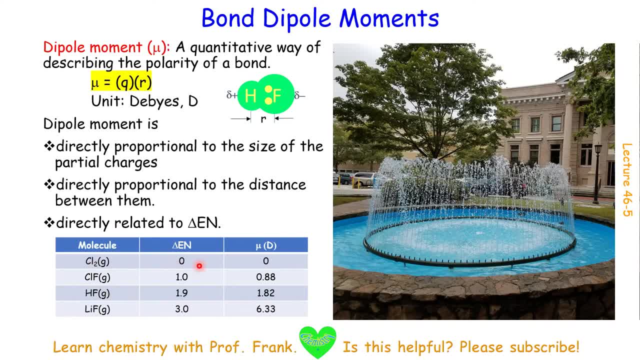 Chlorine molecule- data EN is 0,. dipole moment is 0,. no dipole, no dipole moment. Chlorine fluoride: data EN equals 1, then the dipole moment is 0.88 divided. 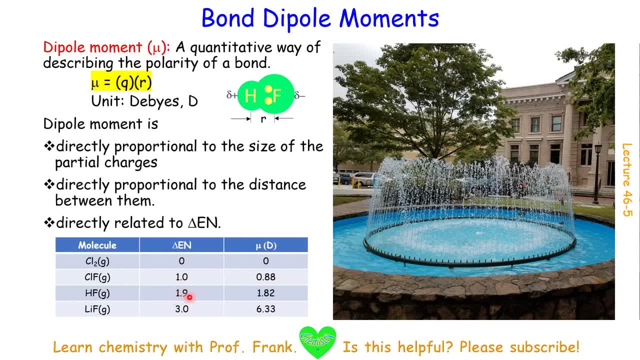 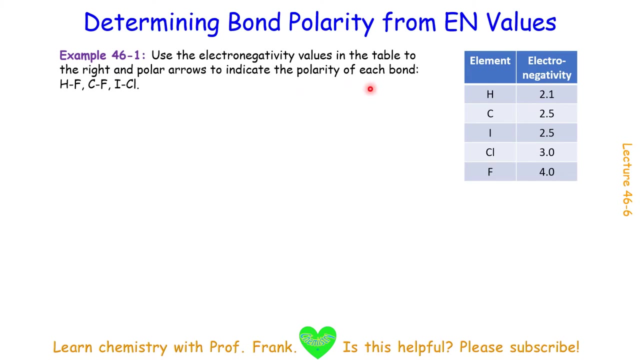 When data EN is increased to 1.9, as in HF molecule, the dipole moment is also increased. That's the relationship between data EN and the dipole moment. Let's use the electron negativity values in this table to indicate the polarity of each bond. 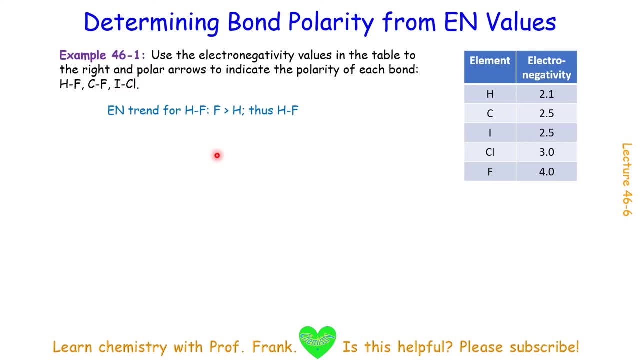 We have three bonds here. Let's take a look at the first one. The electron negativity trend for hydrogen and fluorine Chlorine is more electron negative than hydrogen. Therefore this HF bond has a polarity With a partially positive hydrogen end and a partially negative fluorine end. 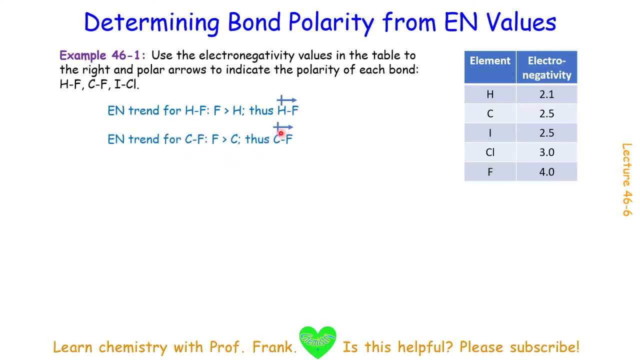 For CF bond, the carbon end carries partially positive and the fluorine end carries partially negative charge. Thus the electron negativity for iodine is smaller than the electron negativity for chlorine. Therefore the iodine end of the ICl bond carries partially positive and the chlorine end carries partially negative charge. 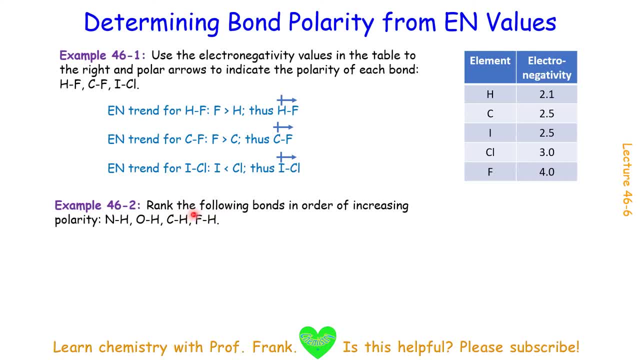 The second example. we need to rank those following bonds in order of increasing polarity, Because all bonds, if you take a closer look, contain hydrogen and hydrogen's electron negativity is smaller than all of the other bonded atoms. the trend in data EN should be the same as the electron negativity trend for the four other bonded atoms. 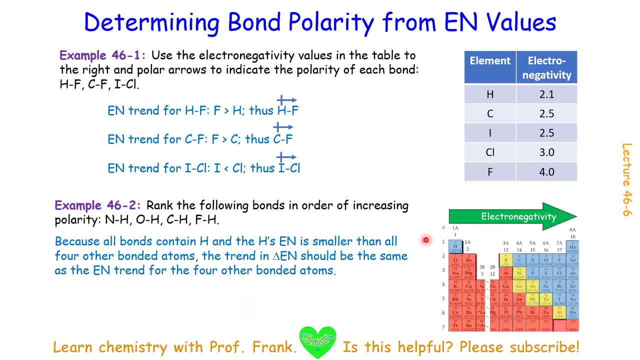 nitrogen, oxygen, carbon and fluorine. We use the electron negativity trend learned previously. The electron negativity for the four other atoms: Fluorine has the highest electron negativity, followed by oxygen, the nitrogen and carbon has the lowest electron negativity. 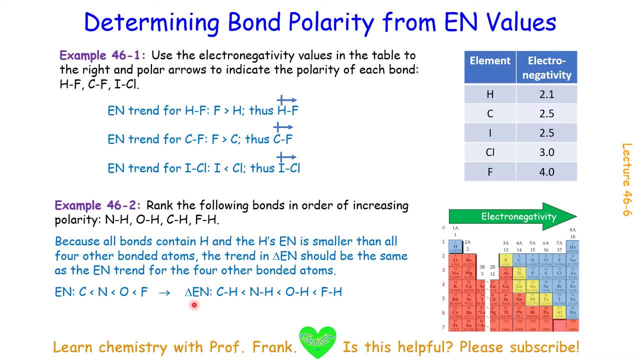 Therefore, the trend in electron negativity difference for those four bonds should be: CH bond has the smallest data EN value, while FH bond has the largest data EN value. Therefore, the bond polarity trend should be CH bond, as the same as the electron negativity difference trend here. 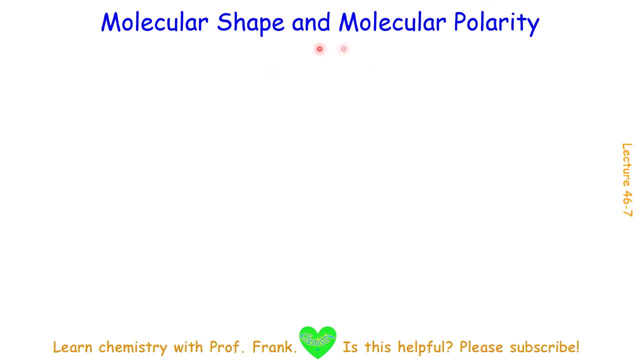 Now let's take a look at the polarity of molecules. When data EN between two atoms is greater than zero, then the bond between them has a certain degree of polarity. The larger the difference in electron negativity, the greater the polarity of the bond. 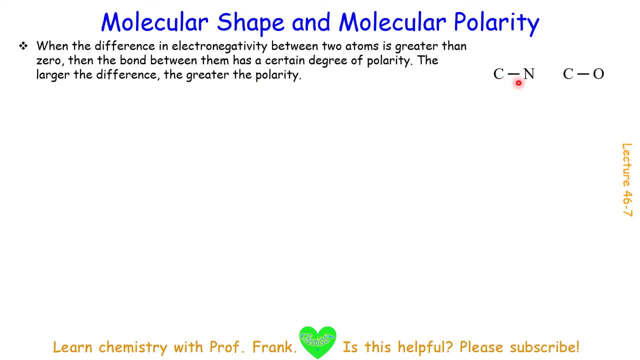 So you can see here carbon-nitrogen bond and carbon-oxygen bond. The bond dipole shows the nitrogen end carries partially negative charge And for this CO bond. this is the direction of the dipole moment, Since the electron difference in CN bond is smaller than the electron difference in CO bond. 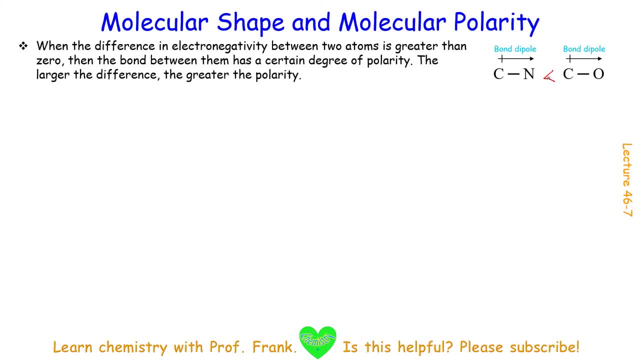 the polarity of the CO bond should be greater than the polarity of the CN bond. That is because the greater the difference in electron negativity, the greater the polarity. If the molecular shape is symmetrical and all surrounding atoms are the same, then the molecule is non-polar. 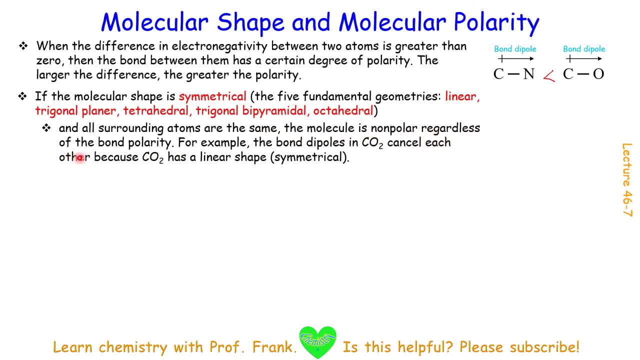 regardless of the bond polarity. Let's take carbon dioxide as an example. You may say: oh yeah, the CO double bond, they are polar bonds. Therefore, this molecule should be polar. Yes and no. Yes, the CO double bonds are polar bonds. 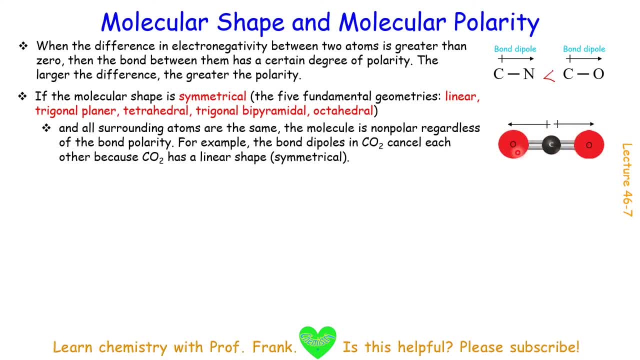 No, this molecule is non-polar. Why? Because the dipole moment of the two double bonds here has the same amplitude but different directions. So therefore, the dipole moments of the two bonds, they are canceled and that leaves the molecule non-polar. 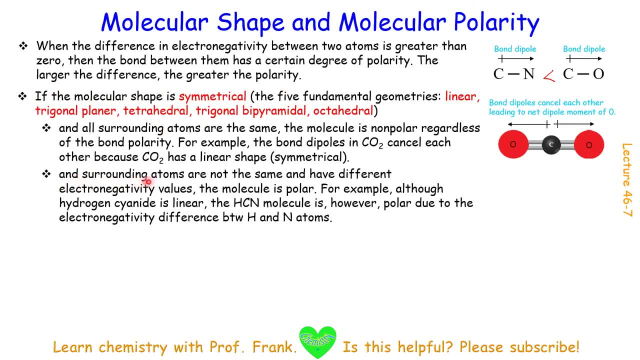 If the molecular shape is symmetrical and surrounding atoms are not the same and have different electron activity values, the molecule is polar. For example, although this hydrogen cyanide molecule is linear, but the HCN molecule is still polar. Why? 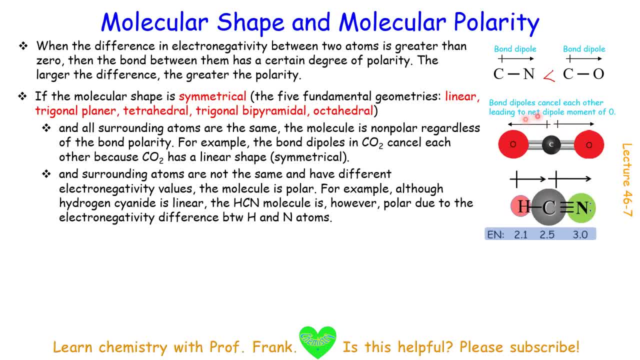 Unlike here, the dipole moments are canceled. Here there is a net dipole moment. The right end carries partially negative charge. If the molecular shape is asymmetrical, the molecule is polar, regardless whether the surrounding atoms are the same or not. 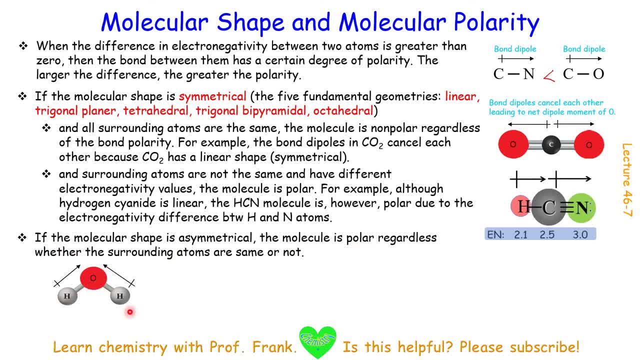 For example, water has a bent structure that is not symmetrical. The symmetrical structures are only the five fundamental geometries: Linear, trigonal, planar, tetrahedral, trigonal, bipyramidal or autahedral. So one is not one of those five fundamental geometries.